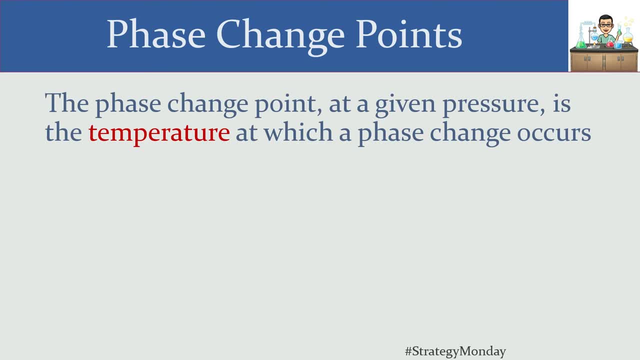 pressure is going to be the temperature at which that phase change happens, And so the substance then, because the phase change is happening at that temperature, it's not happening below the temperature, it's not happening above that temperature, it's happening at that particular. 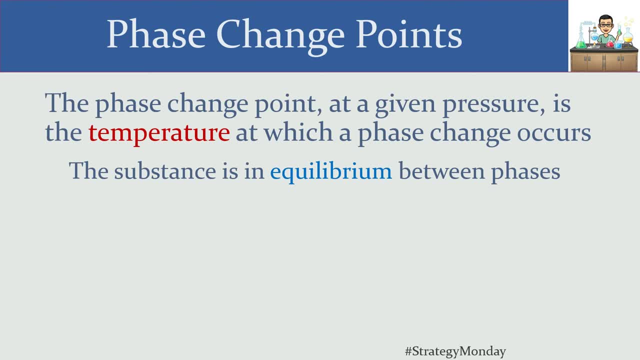 temperature. That means that the substance needs to be in equilibrium between phases, right When you're crossing a border between one city and another, or between one county and another, technically that border doesn't belong to either side, So you're not really in one city, you're not. 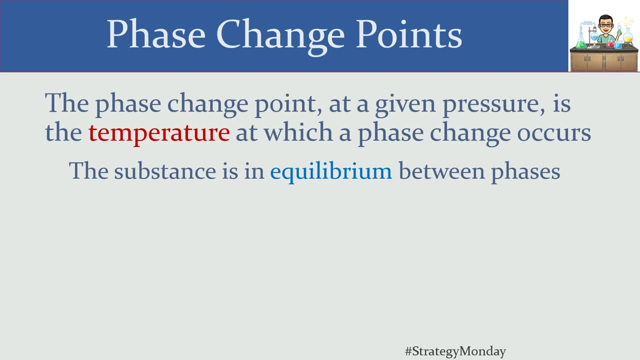 really in another. the border, that imaginary line, doesn't belong to either side, it's right between, And so when we're right at that phase change point, it means that we're not really one phase, we're not really another. we could be either or right- And if we're getting literal here- right, driving in a car on a border. 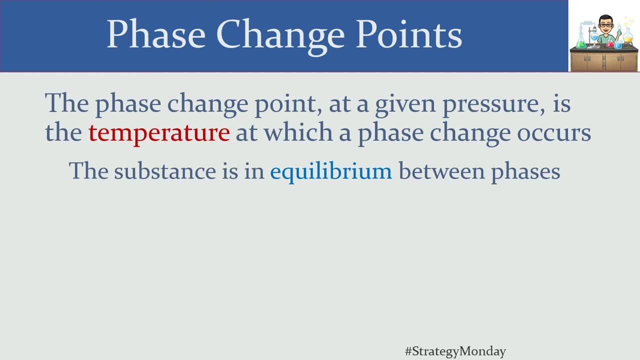 between cities. a portion of your car is in one city and a portion of your car is in another city. you're not really in one city or another, you're kind of in that in-between zone, And so a substance is in equilibrium between phases whenever it reaches that phase change point, And so for. 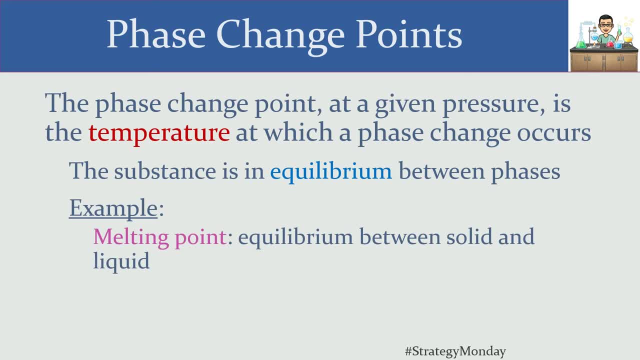 example, the melting point represents the following: If our ice cube is melting, it means it's transitioning over from solid to liquid. So that means that at the melting point that water is in equilibrium between the solid phase and the liquid phase. So let's say we take another phase transition. So let's say we're 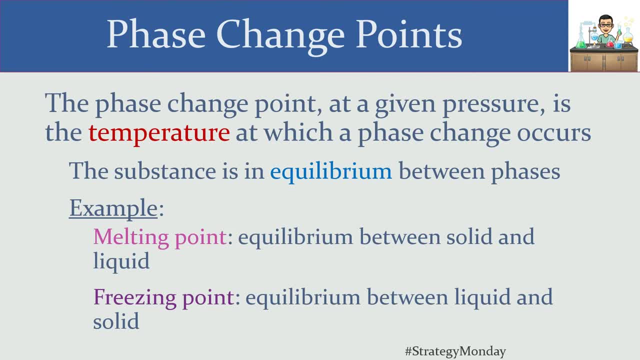 talking about freezing instead. So freezing, when a substance freezes, it goes from liquid to solid. So that means that I am going from liquid water to ice and the freezing point is the point at which I'm in equilibrium between the liquid and the solid phases. So if you pause and take a look at the two, 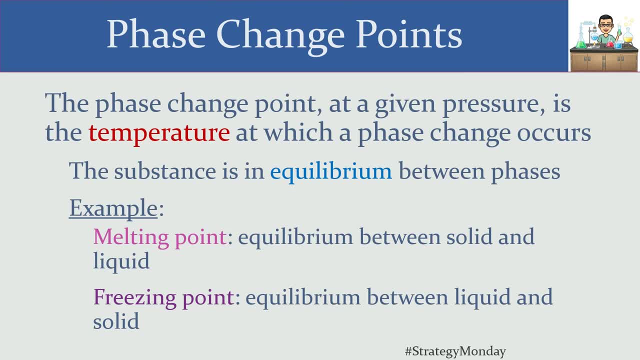 statements that we just mentioned, how we described the melting point and how we described the freezing point. you'll notice I said the same thing for both right. In both those instances I said: we're equilibrium between the solid and the liquid phases And the conclusion we can logically draw. 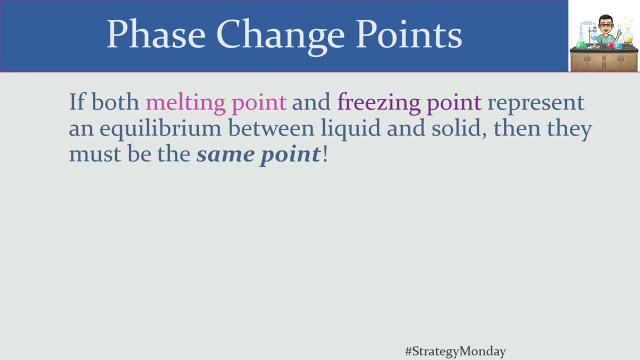 then, is that, because the melting point and the freezing point represent an equilibrium between liquid and solid, they must be the same exact point, And you want to be able to draw an equation that you already know, that intuitively. For example, since we keep talking about water, the melting, 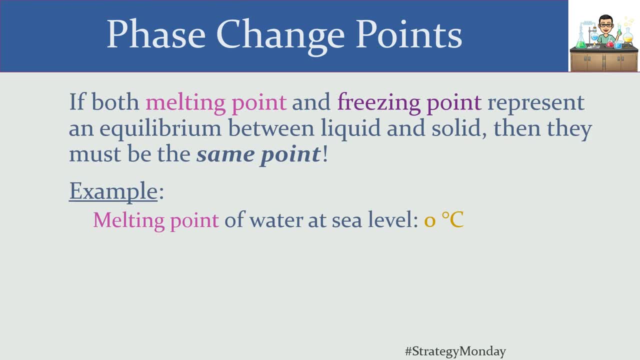 point of water at sea level is zero degrees Celsius, But you also know that the freezing point of water at sea level is zero degrees Celsius. So anytime you have opposite phase changes, strategically you can always think of them as the same point right? So on an exam, if you're given the melting point of 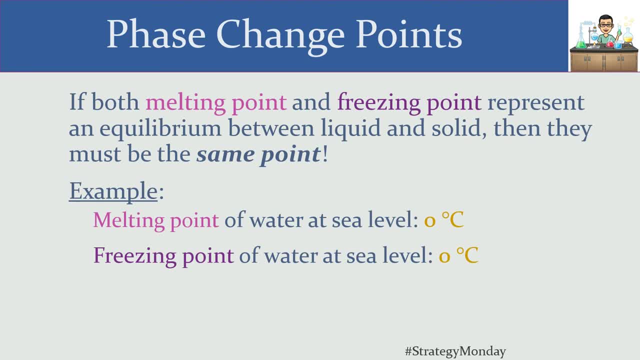 a substance, you don't need to be given the freezing point. You should already know what the freezing point is. It is indeed the melting point, And so whenever we're talking about opposite phase changes strategically, you want to think about them as the same exact point. And if certain changes occur to one of 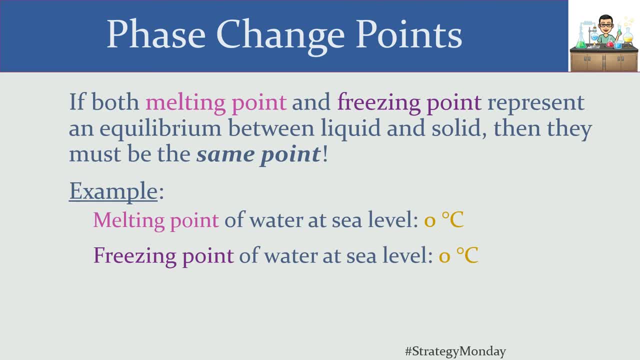 those phase change points, it must be happening to the other. So one of the things that we talked about in terms of colligative properties is that we took a look at freezing point depression. Well, I could have easily just said melting point depression, because the freezing point and the 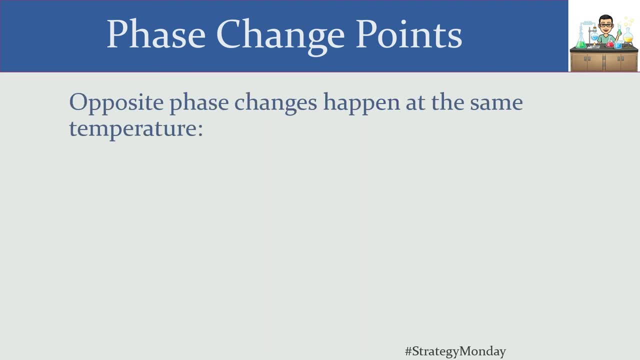 melting point aren't the same exact thing, So opposite phase changes are going to happen at the same temperature. We already saw that with melting and freezing point. We can also extend that to the other pairs of phase changes. So, for example, the boiling point of water you know to be 100. 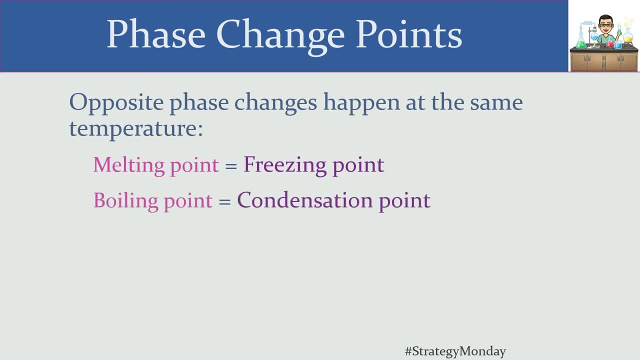 degrees Celsius. Well, that means that you also know the condensation point of water is identical to it, and it's also 100 degrees Celsius. So, again, you don't need to be given the temperatures of each of the phase changes in detail. All you need to be given is one, and then you can figure out what. 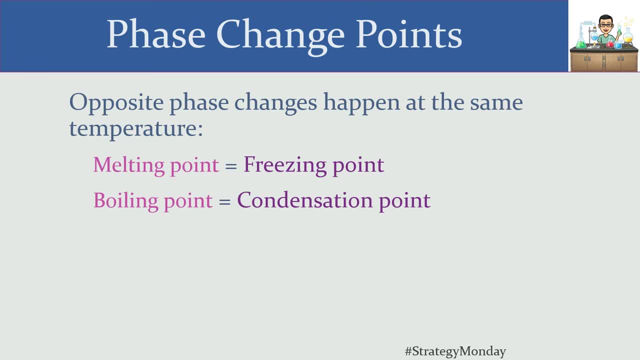 the condensation point is for the opposite phase change. It's the exact same thing. And if you're at a point at which your substance can sublime, its deposition point is exactly the same. So opposite phase changes. they occur at the exact same temperature And a similar phenomenon happens. 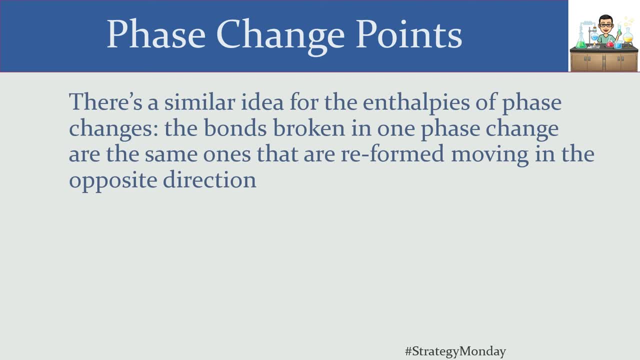 with the enthalpies of phase changes. And so when you go through and you measure how much energy is required to be able to break down a mole of a substance, well, whether you're breaking bonds right, The bonds that you break are the same ones that you're going to have to reform. 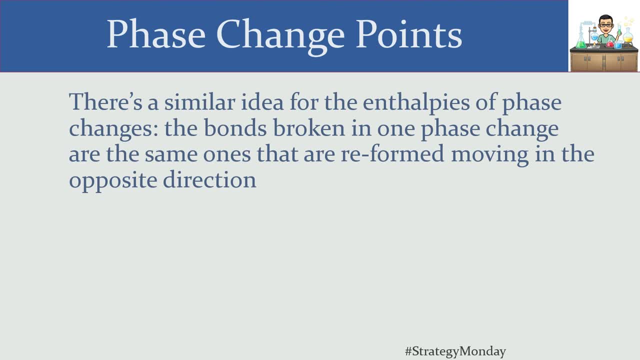 And going through the opposite phase change. So, for instance, when you're melting stuff down, you got to break bonds in order to take that solid into the liquid phase. Well, if you go from liquid back to solid, you have to reform those same bonds that you broke.